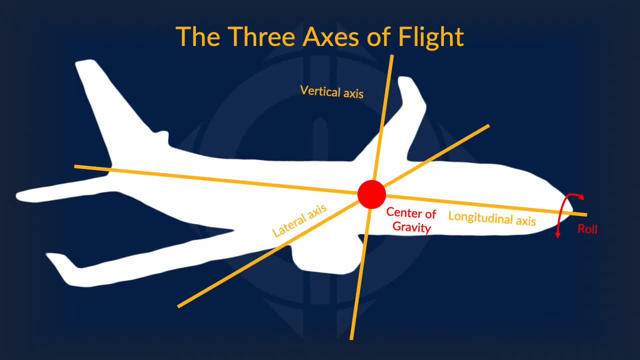 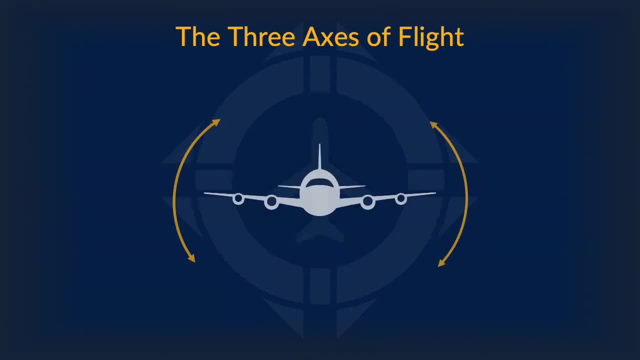 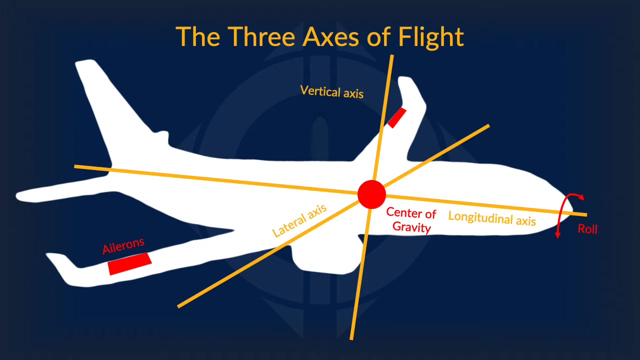 video. Our next axis of rotation is the longitudinal, For which the rotation is termed a roll. Here is a quick demonstration of a roll using the front view of the airplane. The ailerons control rotations about the longitudinal axes and allows a pilot to roll clockwise or counterclockwise. Rolling plays a crucial part in the turning of 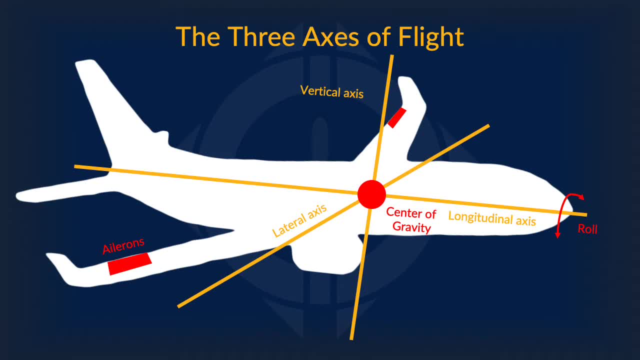 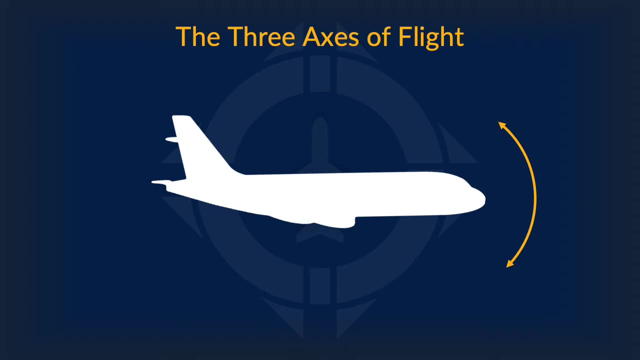 the airplane, which we'll get to in our next video. Last but certainly not least, we have rotation about the lateral axes, for which the rotation is named pitch. Here is again a quick demonstration using the side view of an airplane. 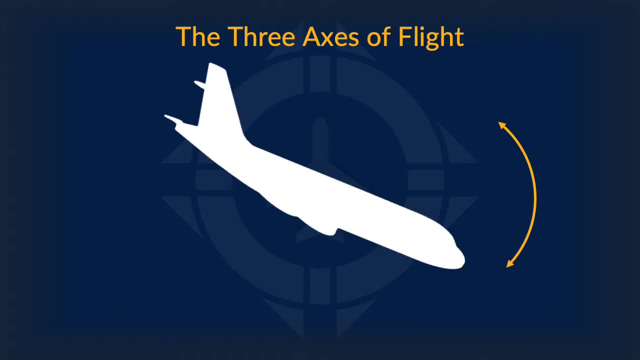 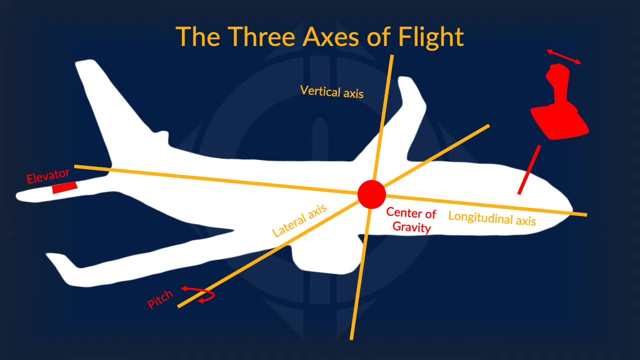 A pilot can pitch an airplane up or down through the elevator, which alters the direction of airflow past the wing, to generate more or less of the same air flow. This is because the ailerons are low and the aeroroyal power is located as low as a given When the aileron is at the height of the plane and the plane is at its limit. it's usually a good thing to lift an aeroroyal power a little bit to prevent it from crashing. And then here is a test lift at the back of the aircraft. Many of us may have a good. 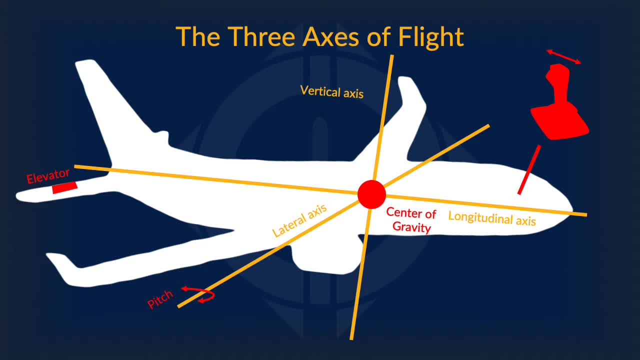 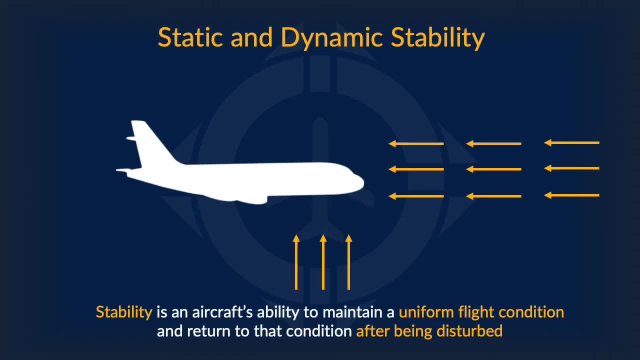 mental image of the joystick used in commercial aviation, and this is its role: to control the elevators. Now we move onto something more interesting: stability. Stability is simply an aircraft's ability to maintain a uniform flight condition and return to that condition after being disturbed. 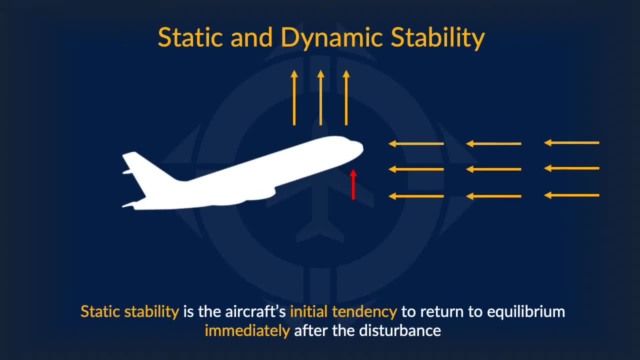 Stability is split into two types: stability and stability. Stability is split into two types: static and dynamic. Static stability is the aircraft's initial tendency to return to equilibrium immediately after the disturbance. Alright, but what does that mean? Let's go through how this looks like in a real setting. 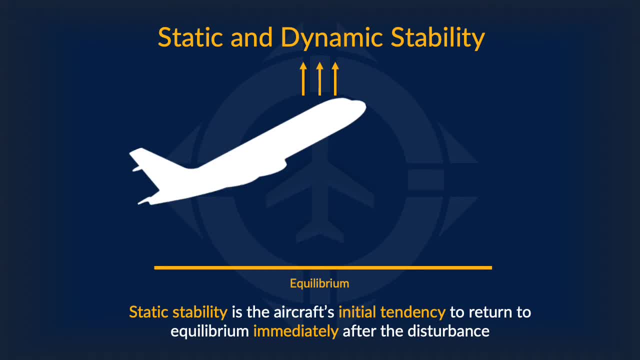 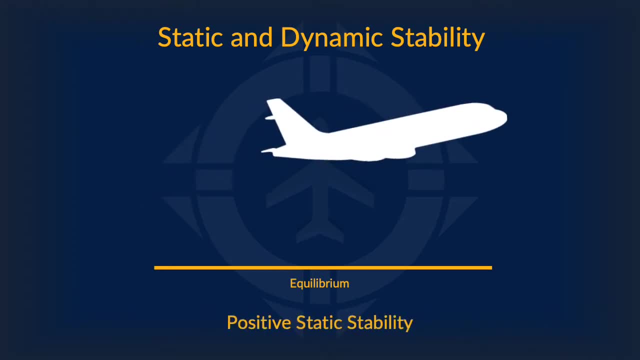 Say, a sudden updraft pushes an airplane upwards. Static stability shows the action of the airplane immediately after this sudden shift in its pitch. There are three types of static stability, the first of which is positive static stability shown here. It basically means that the airplane has a tendency to immediately self-correct. 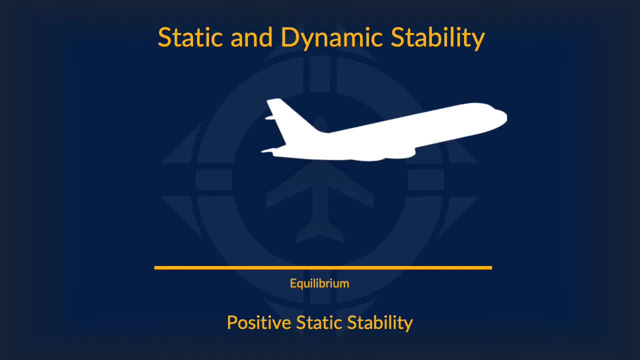 this sudden change Great. This characteristic is highly desirable for airplanes used for tasks such as pilot training or transporting materials. The next type is neutral static stability. Again, the airplane suddenly pitches upwards because of an updraft and it doesn't self-correct. 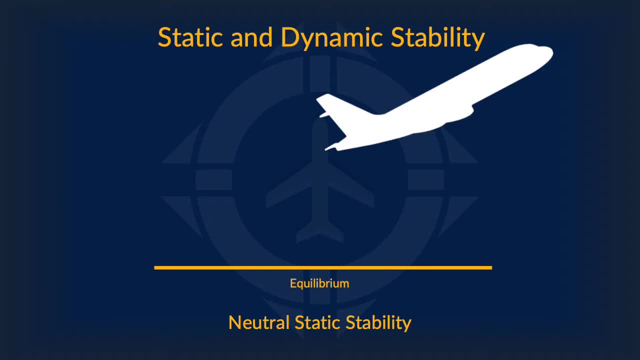 at all. Its pitch stays exactly the same. It's not optimal, but it isn't too bad either. The last type is negative static stability, which, as you may have guessed from the trend so far, means that the airplane actually pitches even more after the sudden change. Let's take 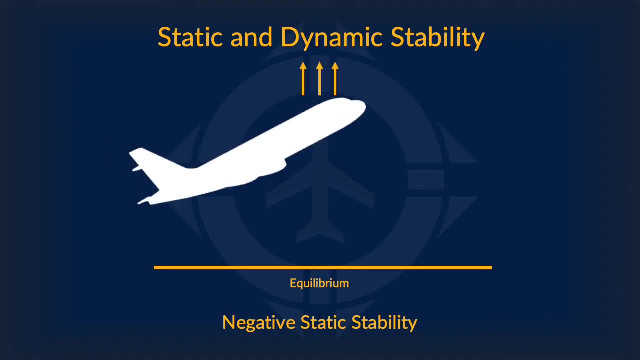 a look. The second type is negative static stability which, as you may have guessed from the trend so far, means that the airplane has a tendency to immediately self-correct. this sudden change, An updraft as usual, And then suddenly the airplane suddenly jerks up even more. This is very undesirable in 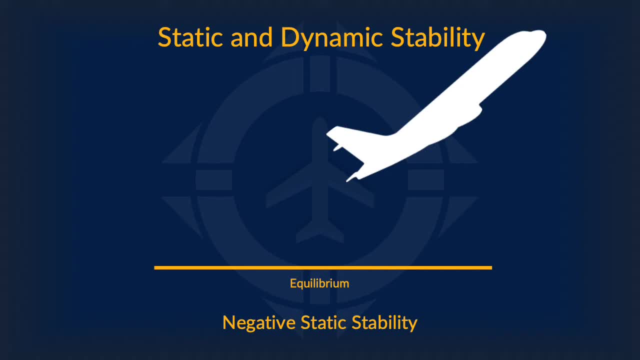 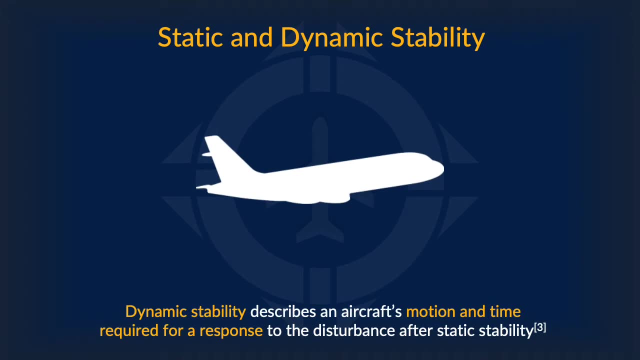 most airplanes, as it greatly increases the risk of a stall if the angle of attack is too high. Dynamic stability, on the other hand, describes an aircraft's motion and time required after static stability. Basically, it describes the airplane's behavior after the initial 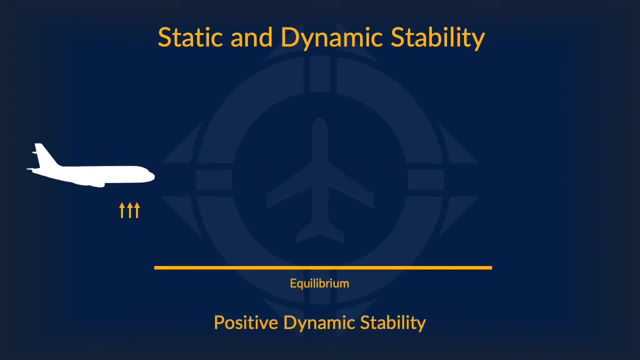 response from static stability. First we have positive dynamic stability where basically, the airplane will self-correct over time. Let's take a look. This is a rough depiction of a theoretical line the airplane will follow if its dynamic stability is positive. As one can see, the fluctuations decrease in magnitude over time. 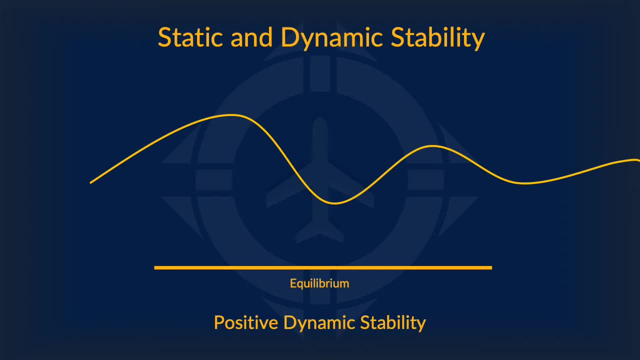 That means, without any external forces or action from the pilot, the airplane will theoretically automatically go back to its undisturbed state. This is very useful for trainer aircrafts as well as cargo planes. Next up, we have neutral dynamic stability. Here is the approximate path a plane with neutral dynamic stability may follow. 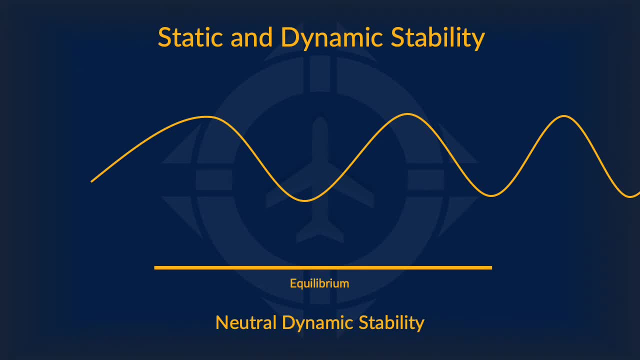 Next, As one can see, the fluctuations magnitude doesn't change at all. Theoretically, this means that the airplane will fly on forever, fluctuating at this exact magnitude and speed forever. Lastly, we have negative dynamic stability. Here is the path, as before. 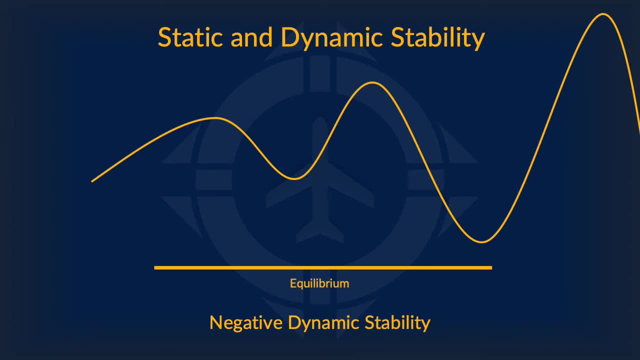 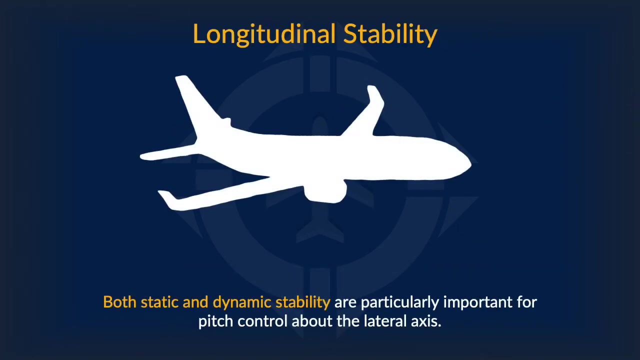 As one can see. Next, As one can see, the fluctuations actually increase in magnitude over time. This is very undesirable for most airplanes as again, it could be difficult to regain control and could quickly lead to a stall and a crash. Both types of stability are particularly important for pitch control over the lateral axis, which 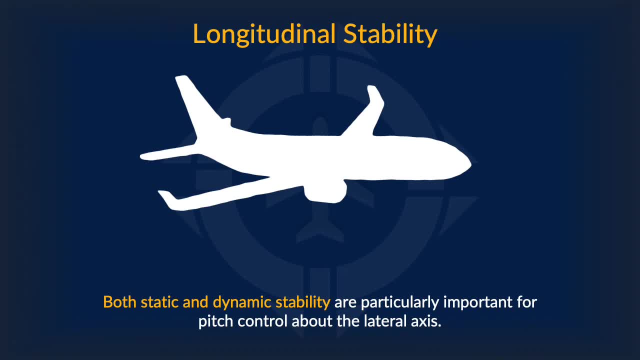 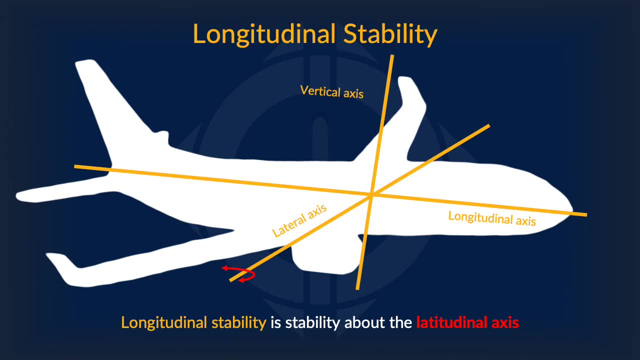 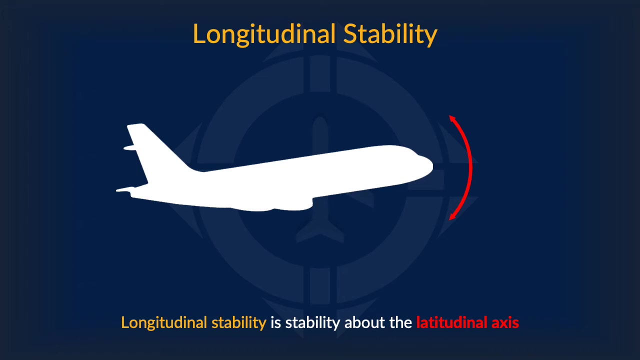 is what we explored just now with the fluctuations looking at the side view of the airplane. Next, Next, Stability about the latitudinal axes. Yes, you heard that right. Longitudinal stability is stability about the latitudinal axes. So how can we improve the longitudinal stability of an aircraft? 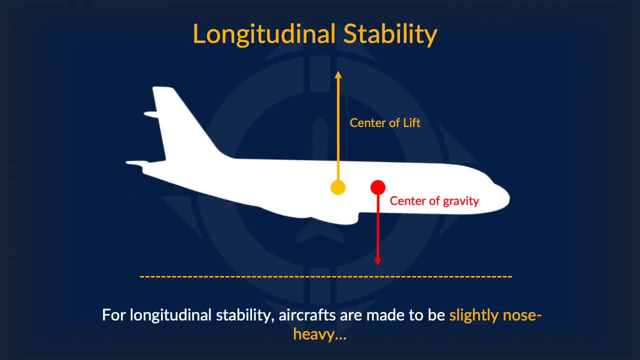 One thing aircraft designers do is they actually make the aircraft slightly nose-heavy. Now, this would usually be undesirable, as it means that the airplane has a tendency to flip forwards due to the distance between the center of lift and the center of gravity. So to offset this, the horizontal stabilizer at the back of the airplane has a slightly negative angle of attack. 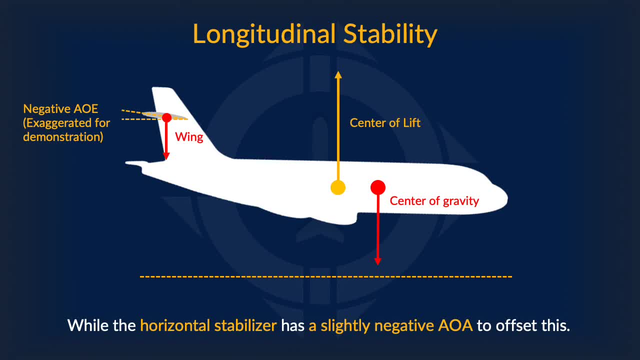 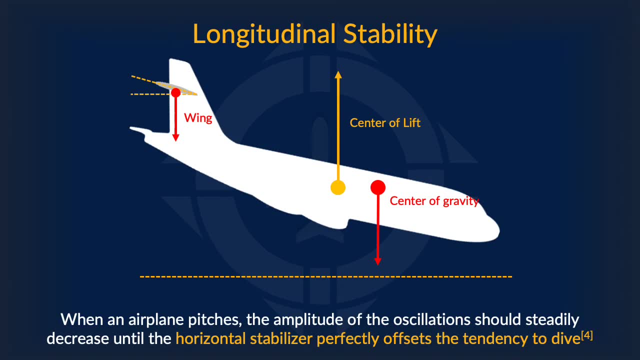 This provides another source of weight, or negative lift. in this case, that cancels out the tendency to nosedive. So what does this do? Well, when an airplane pitches suddenly, the amplitude of the oscillations would steadily decrease Until the horizontal stabilizer perfectly offsets the tendency to dive. 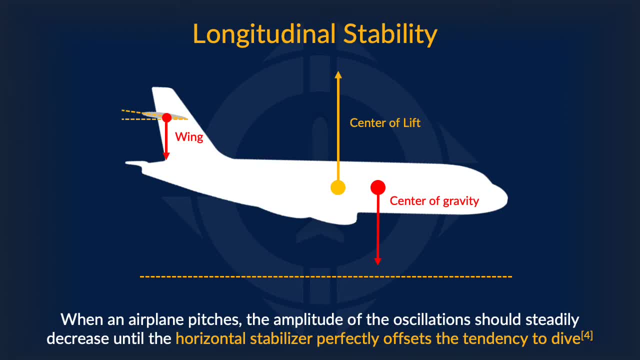 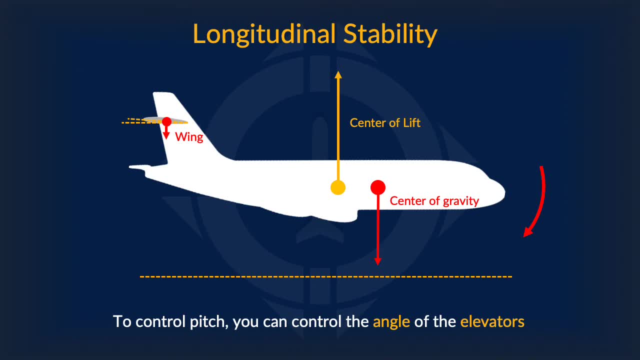 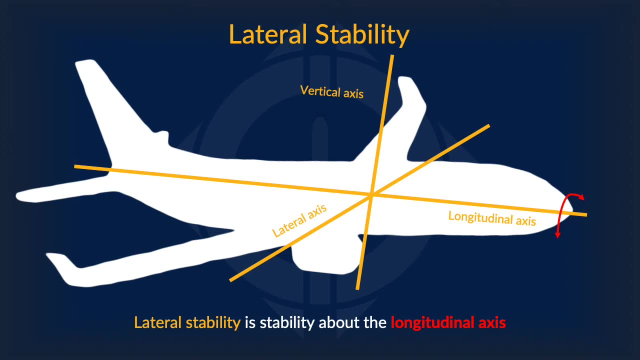 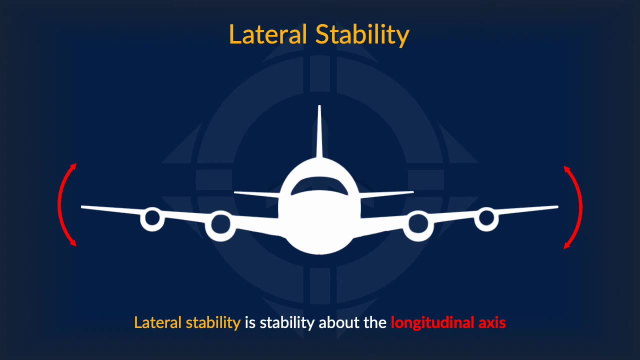 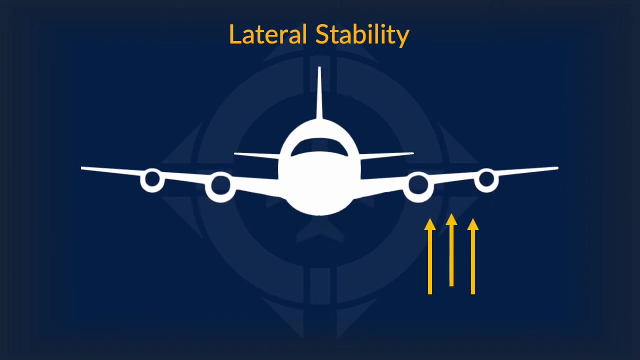 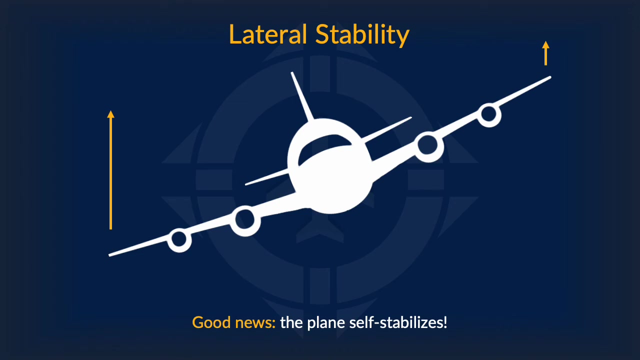 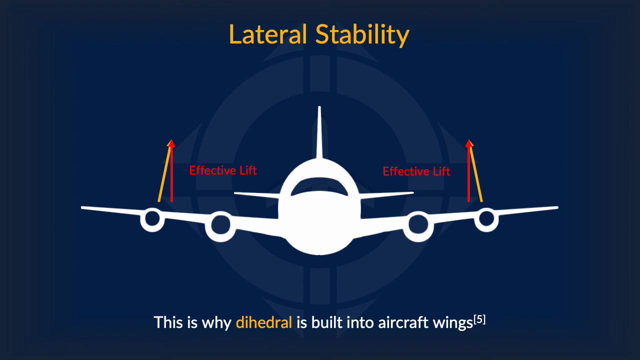 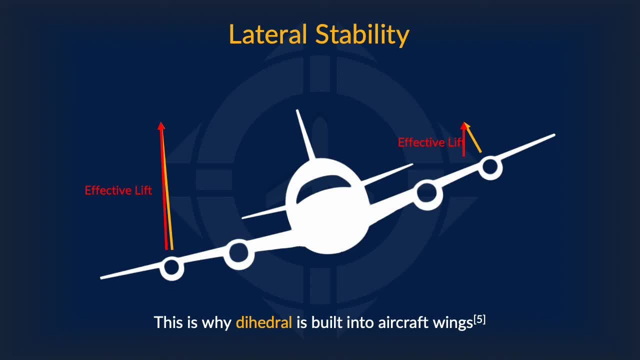 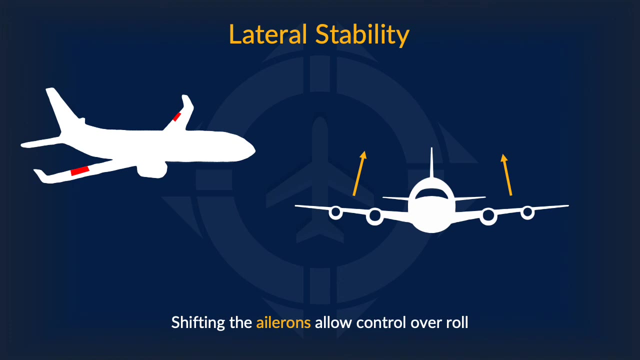 while the outer wing's vertical component decreases. This allows an aircraft to self-correct much more easily, Great Okay. in case it's not enough, though, shifting the ailerons enables control over roll, as we have stated before. How this works is that through shifting one aileron downwards. 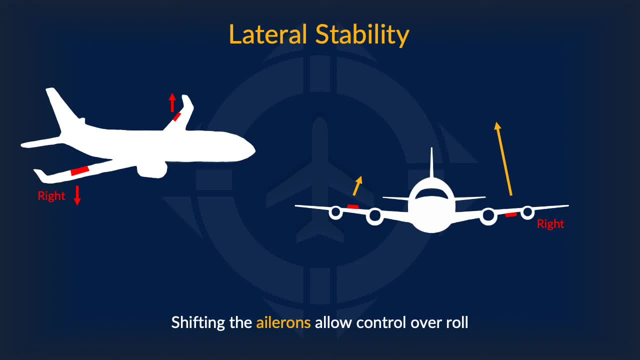 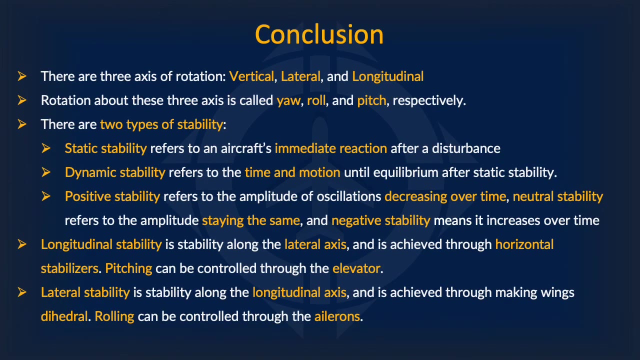 while shifting another one upwards, the lift vectors can change. How this exactly works will be explored in our next video, And so shifting the ailerons gives you control over the roll. So here's a quick recap of what we learned today.